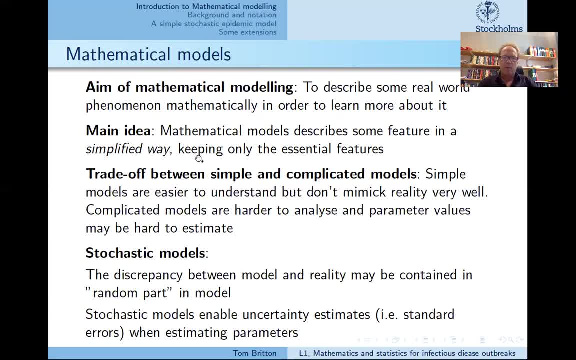 So a mathematical model is always a simplification of the real world phenomenon. But the question is: how much do you want to simplify? And there is a trade-off between making the model very simple or slightly more complicated. The advantages with having a simple model is that they are quite often easier to understand and analyze. 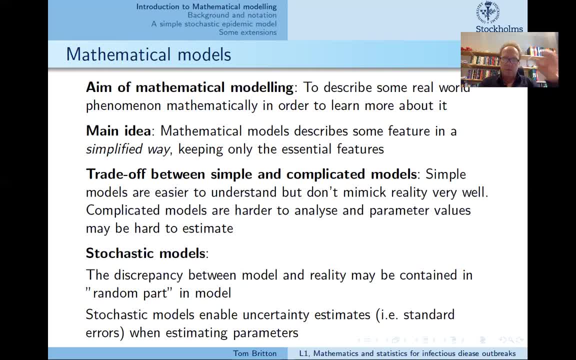 But the downside of them is that typically they don't mimic reality as well as more complicated models. So if you have a too simple model, you might not catch the important features of the thing you're interested in. Complicated models, however, they can capture reality better. 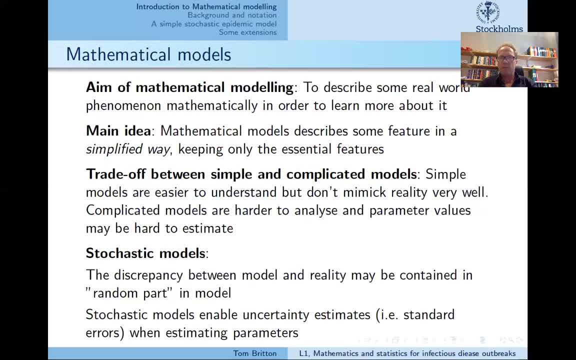 In the sense that if you have more features in your model, you might capture reality better. But the downside of complicated models is that first of all, they're harder to analyze, But using numerics this is quite often possible. But another downside is that 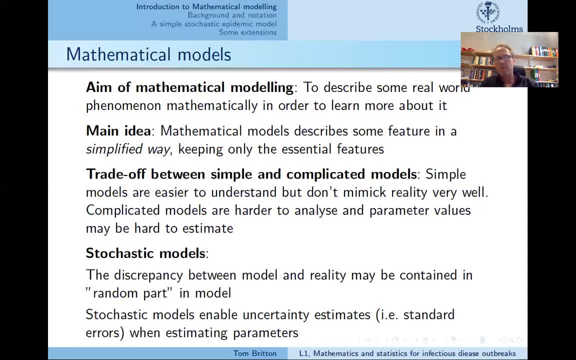 when you insert parameter values, for numerical values for the parameters- typically a complicated model has lots of parameters- Then you have to say: if you want to say something about reality, you have to give numerical values to all these parameters. And to know what are sensible parameter values is very hard. 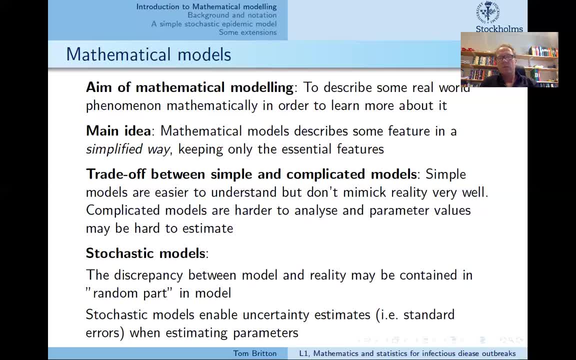 And if you give wrong parameter values, your conclusions might not be valid. So that is the downside of complicated models. So I promote using both So typically. you might start with a simple model, which you understand better, but it does not capture all the important features. 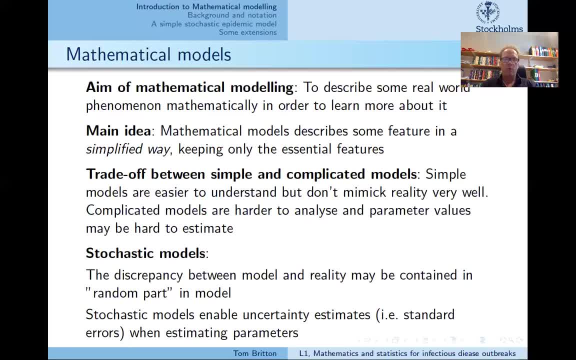 And then you also combine that with a more complicated model to try to mimic reality better, And hopefully you know something about the numerical values of parameters. There will be some Part of this course will be able to do stochastic models, which is within the class of mathematical models. 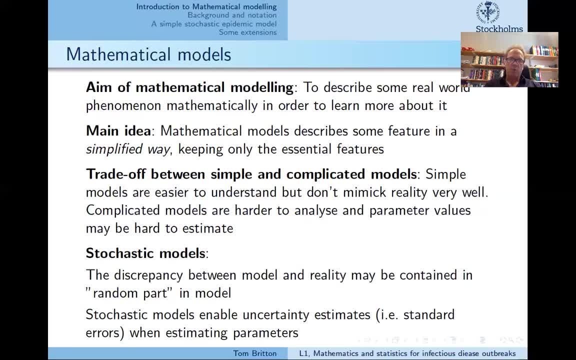 But many people think of mathematical models as deterministic models. But mathematical models could be either deterministic or stochastic. But what is the advantage with stochastic models? There are some advantages and some disadvantages. The advantages are, for instance, that your model does not capture all the features in reality. 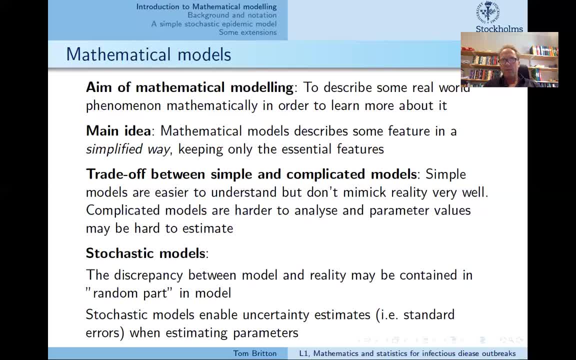 And one way to interpret the randomness in the model is to make that include the things that you do not know in the model. So the random part in the model are those things that are not captured in the model, In the sense of discrepancy between the model and reality. 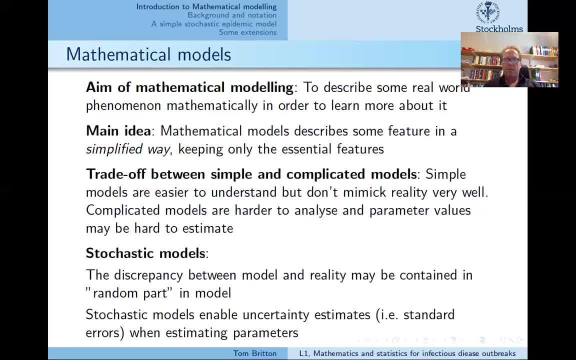 Another advantage with stochastic models is that quite often you want to state something about your conclusions, but also with some measure of confidence, And stochastic models allow for uncertainty estimates, which is a big advantage for them, And a disadvantage with them is, of course, that you 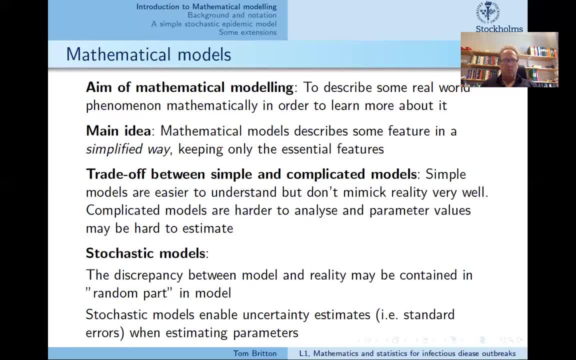 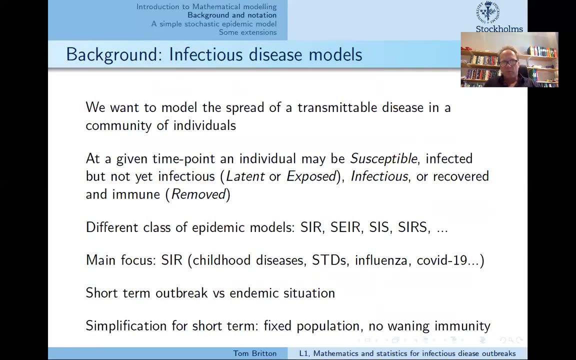 You. They are much harder to analyze. So to say something for a stochastic model is nearly always much harder than it is for a corresponding deterministic model. Anyway, this course is about infectious disease models of different sorts, So we should have in mind that we want 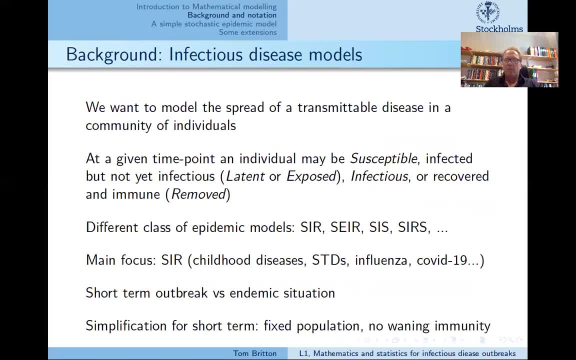 We now want to model the spread of some transmittable disease in a community of individuals. We will mainly talk about human diseases, but it could equally well be diseases among animals, wild or domestic animals, or even plants, But for most of the time we'll consider human diseases. 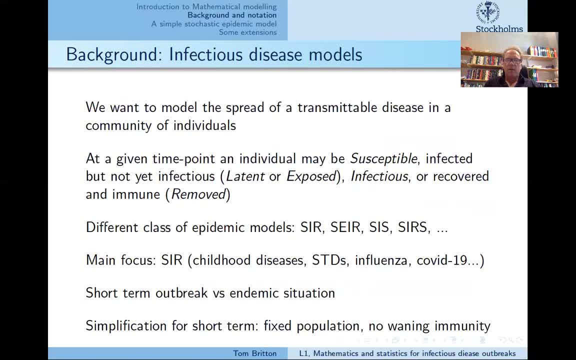 And for such models you can typically classify an individual into different categories. A common categorization is that some individuals are susceptible. other individuals have been infected but they're not yet infectious. That state is often called latent or exposed. Another class state is that you are infectious. 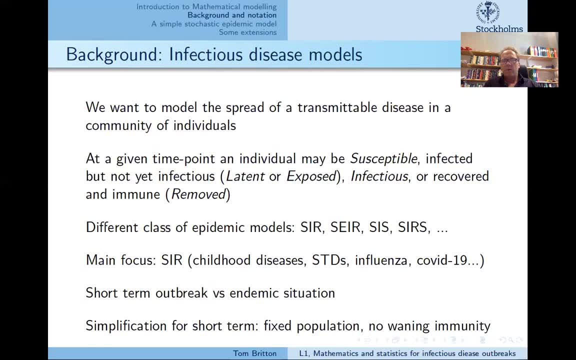 And after some time in the infectious state you typically recover and become immune. So the four states here would be susceptible, exposed, infectious and removed, Or this could be removed or recovered And the interpretation is that you have been infected and are now immune. 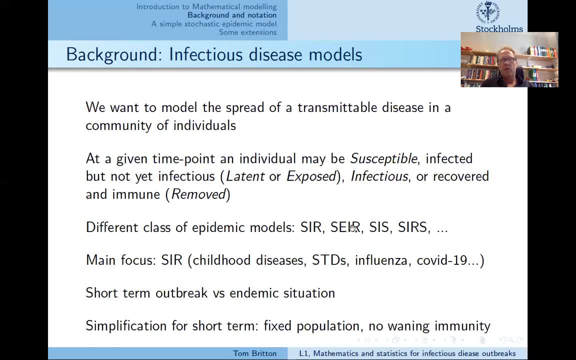 So this class would be called an SEIR epidemic. If you have no latent state or exposed state, it would be an SIR model. If there is no immunity after you recover from the infectious state, you go back to being susceptible. Such a model is called SIS. 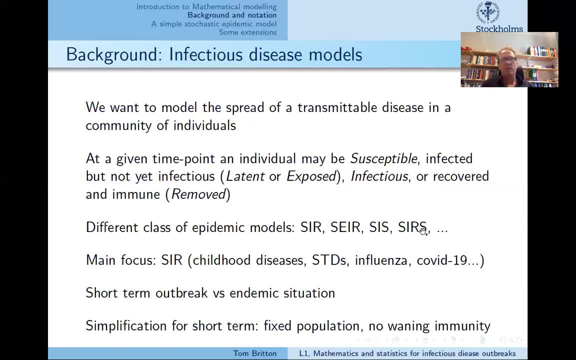 SIR is if you are immune for some time but then go back to susceptible and so on. We will mainly talk about SIR diseases in this course, but also some others. There are a lot of different types of SIR diseases, Of course, if it's an SIR or SIRS. 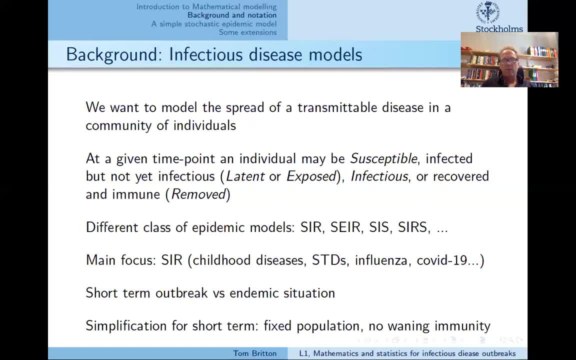 it depends on what time horizon you're looking at Childhood diseases like measles. if you're going to be immune for the rest of your life. With COVID-19 and influenza, that's not the case, but maybe you were immune for a couple of years. 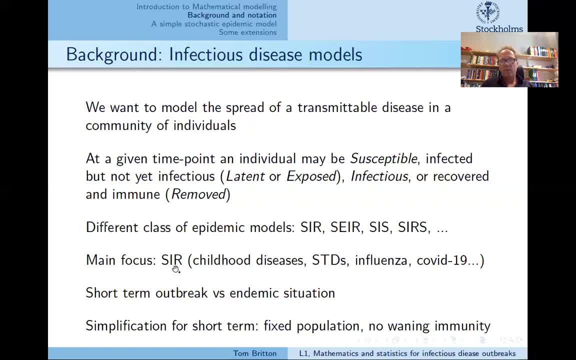 So they would be called SIR models, if you consider a time horizon of a year, let's say. And then you have sexually transmitted diseases which are also SIR or possibly SIS. For instance, chlamydia is considered to be an SIS model. 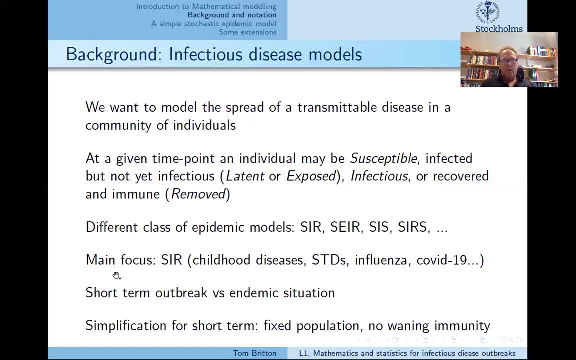 So it depends on the disease you're thinking. What model to use depends on what type of time horizon you're looking at. So if we look at short-term outbreaks or if we look at long-term situations, and then you might be considered. 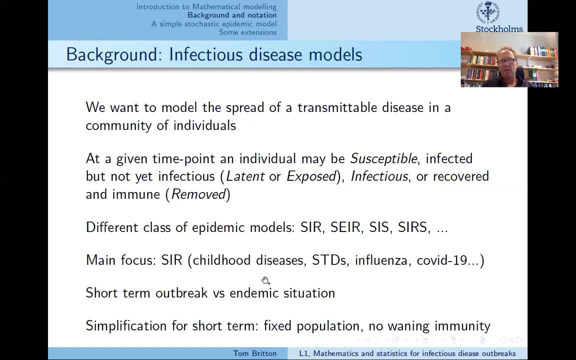 will this disease become endemic, meaning that the disease is present in the community the whole time, or will it disappear after a couple of months or so? If we're interested in a short-term outbreak, then typically we simplify life in line with the description of mathematical models. 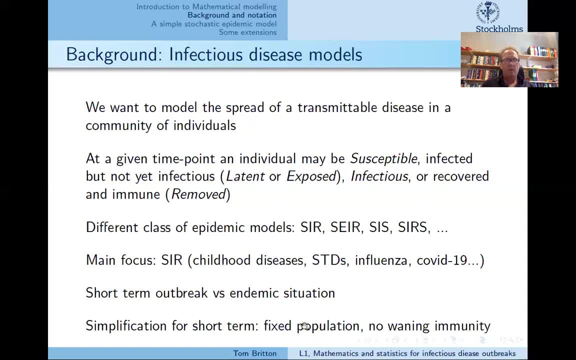 So we assume that we have a fixed population And if we have a short-term outbreak, there is no reason to talk about waning of immunity, Whereas if we look for several years, it's known that for many diseases immunity wanes. 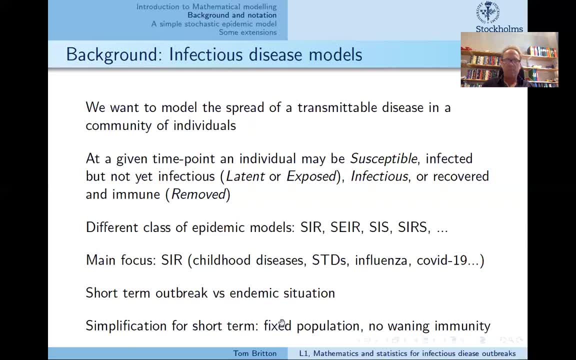 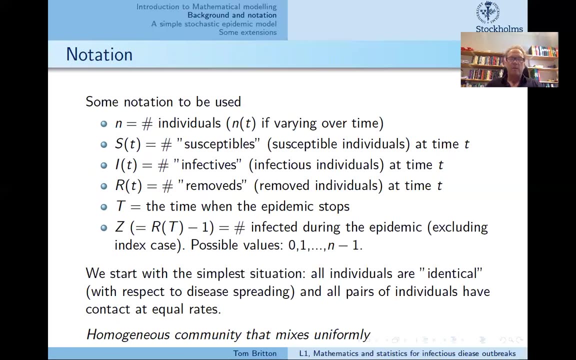 But for short-term outbreaks we consider a fixed population and immunity is 100% during the rest of the study period. So now I will present an SIR, a stochastic model. actually. Before that let me introduce some notation. So we let N be the number of individuals. 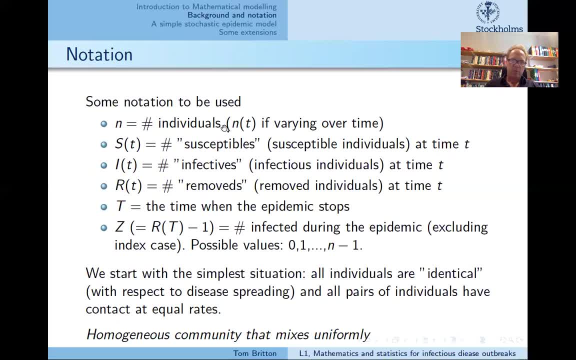 I would consider a fixed population, but if not, it would be called N, so it would vary with time- T is, by the way, time- And this population, or this community, consists of N individuals, and they are classified into either being susceptible: 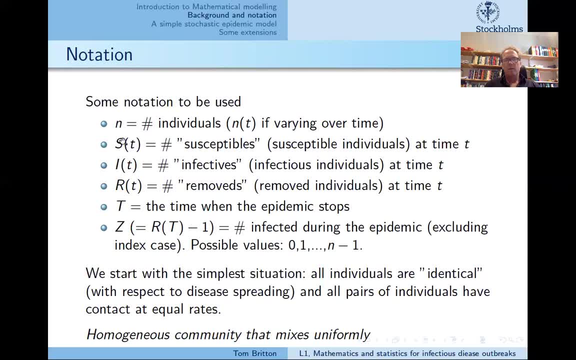 infected and recovered. So S of T is the number of susceptibles at time T, I of T is the number of infectives, meaning infectious individuals, and R of T is the number of recovered or removed at the time T, And these three always sum to N. 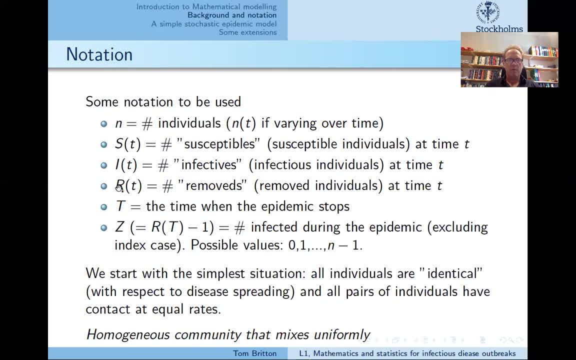 So everyone is either susceptible, infectious or recovered, and you cannot be in both. And then we let capital T be the time when the epidemic stops and we let Z be the number of people that have recovered at the end of the epidemic. But you subtract one. 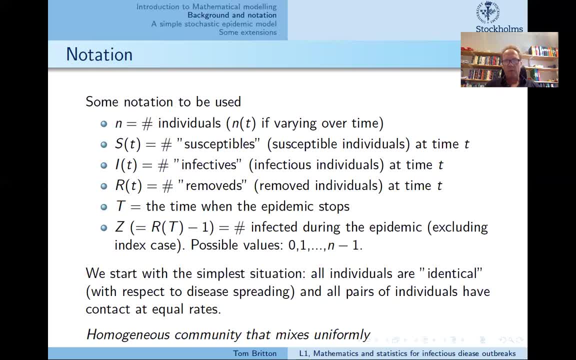 because typically we assume that we start with one single individual infectious and you typically exclude that person. This is not a big issue because we will only be considering N being quite large, so maybe 10,000, and whether we subtract one or not doesn't really matter. 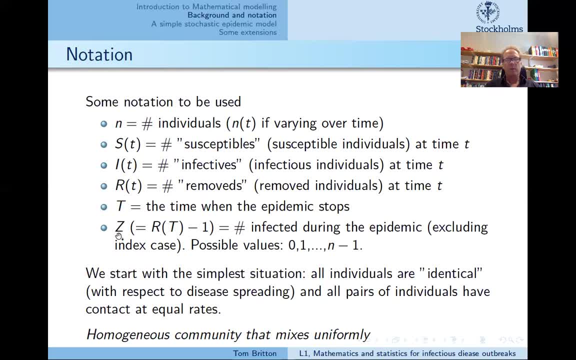 Anyway, Z is the total number of people infected during the epidemic And the possible values, if we exclude the index case would be zero up to N minus one. So if we had 1,000 individuals, the number of people getting infected 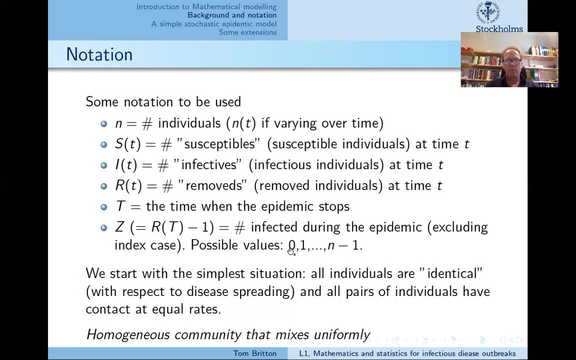 except the index case, the possible values are zero up to 999.. So the first model I will explain is the simplest model, where all individuals behave identically and all individuals are equally susceptible and equally infectious in case they become infected. And also importantly, 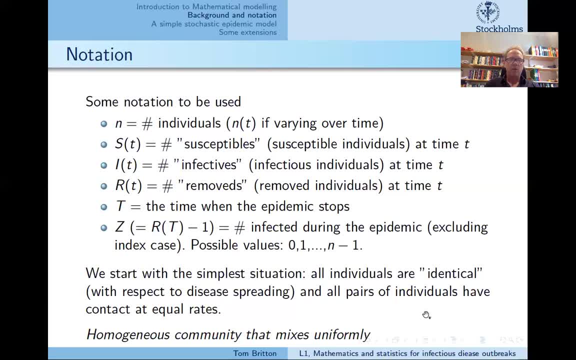 we assume that all pairs of individuals have equal contact rates. so there are no social structures in this simplest model And we have a community, which is called the homogeneous community, that mixes uniformly. Of course this is not realistic, but we start with the simplest possible case. 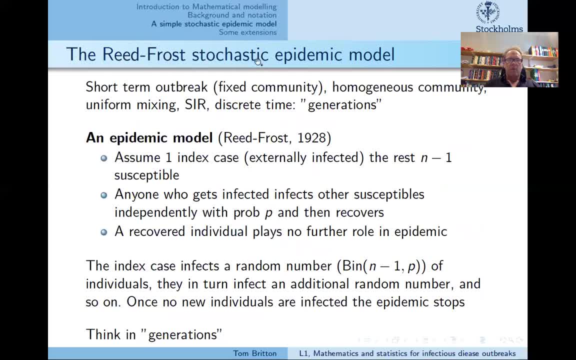 So this model is called the Reed-Frost stochastic epidemic model. So you should think of a short-term outbreak- Perhaps the COVID-19, or an influenza outbreak or something similar- which lasts for a few months or half a year, And here we consider time in terms of generations. 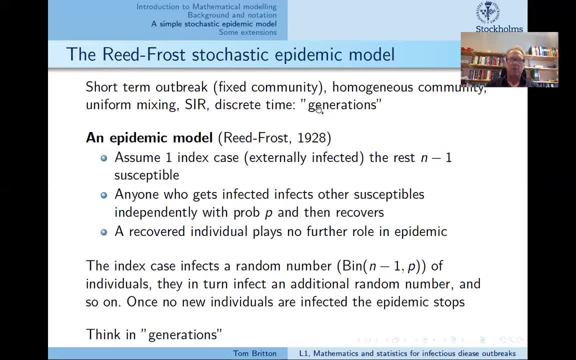 so not really continuous time, but you could think that maybe you're latent for five or six days and you're infectious for a short period, so then you can think of generations. So the model is as follows: We start with one person being infected from outside. 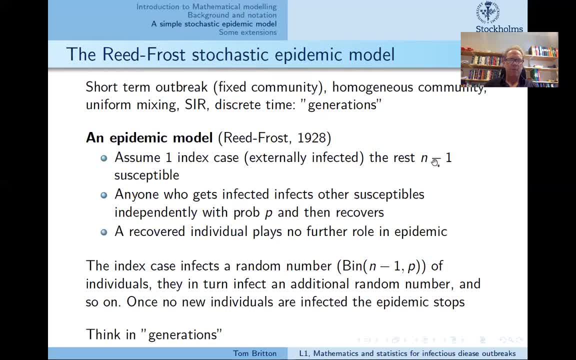 and the remaining individuals are susceptible. And then, during the course of the epidemic, we think of, let's say, weeks. So when we start week one, the index case is infected and everyone else is susceptible. Then week two, some people might get infected. 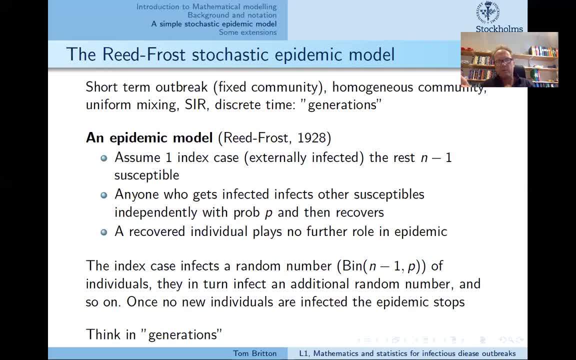 Week three, a different group might get infected And the first group have recovered by then, and so on, And the dynamics are as follows: Anyone who gets infected on some week, the next week will infect each other susceptible individual independently, with some probability P. 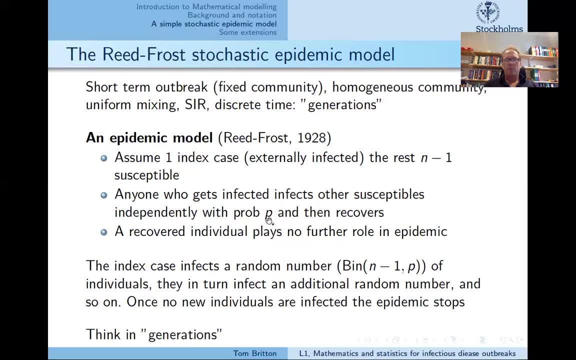 After that you recover. So you can think of that. you have a coin that you toss which comes up with a sign and you decide: infect with probability P and the other side do not infect with probability one minus P. And if you get infected, week 10,. 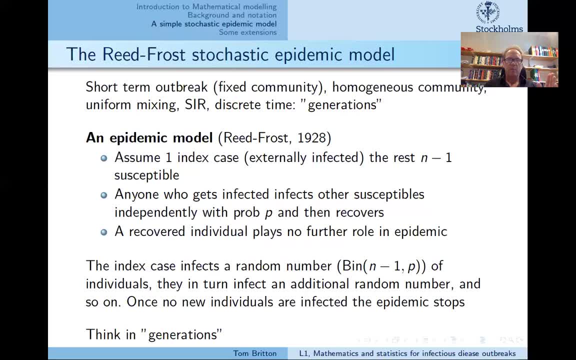 you toss your coins to everyone who is susceptible then and you decide to infect each person. if the coin comes up says infect, and this happens with probability P And then the next time you have recovered and you cannot get reinfected. 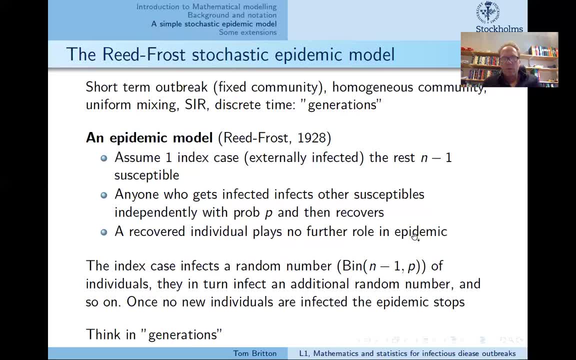 and you play no further role in the epidemic. So week one there was one person infected. Maybe let's say 999 were not infected And suppose P is small. If we have a large community P is typically small, So maybe P is 0.002.. 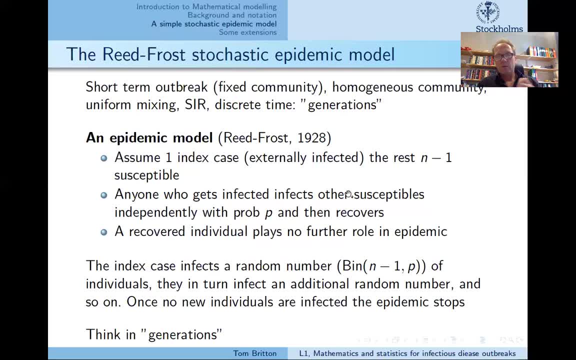 So this index case tosses a coin to each of the other 999 individuals, Infect or not infect, And it's a small chance of infecting. So maybe out of the 909 people that the index case tosses the coin to, let's say that three of those people got infected. 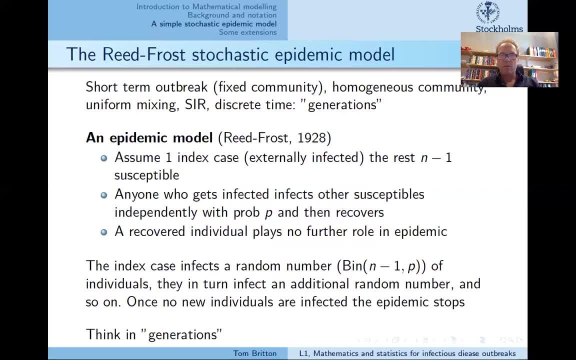 and the other 996 did not get infected, Then that means that week two there are three infected people, The index case has recovered and is by then in the recovered state And the remaining 996 are susceptible. Then the next generation. 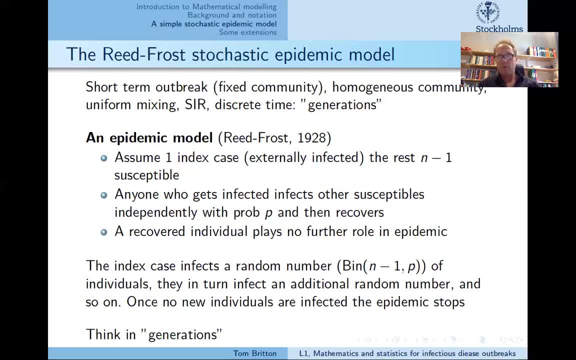 those three individuals. they, each of them, toss a coin to each of the 996 people who are susceptible And infects each one with probability P, So viewed from a susceptible point of view, in week two, in order not to get infected. 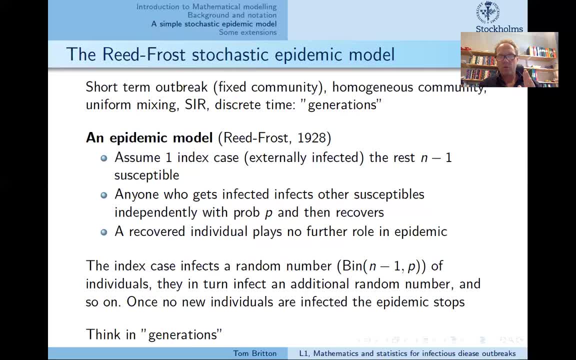 you must avoid the infection coin tossing from each of the three people infected. So it's a bigger chance that you get infected and it's a smaller chance that you avoid getting infected. Anyway, by chance, it could happen that these three individuals 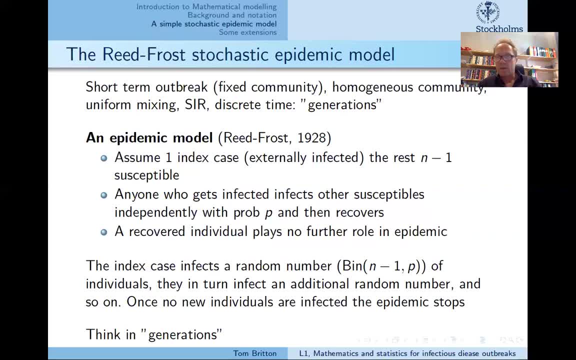 then in the next generation infect, let's say, seven individuals, And then it is the week thereafter. there are then four people in the recovered state, the index case plus the three infected the first generation. There were seven new infected. 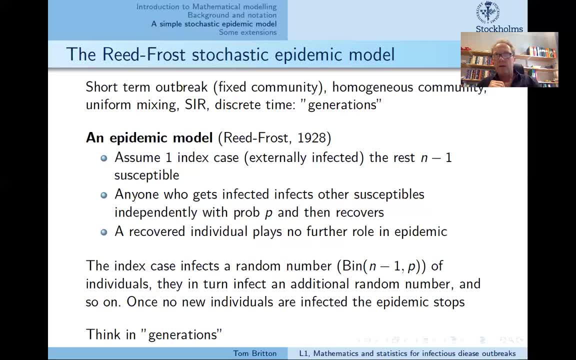 and then there must be 989 susceptible individuals. Then these seven people toss. each of them toss the coins to the 989 individuals to decide whether to infect or not, And each of those 989 individuals escape infection. If they escape, the coin tosses from all the seven individuals. 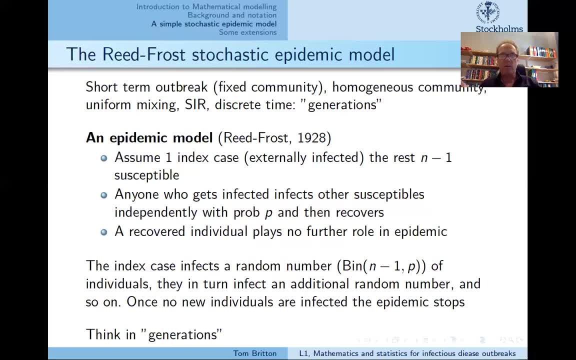 And then this goes on. maybe the next time it was 15 individuals, then the next generation 23 individuals, And this goes on, but the number of susceptible reduces each time, So eventually it will not the number of people getting infected. 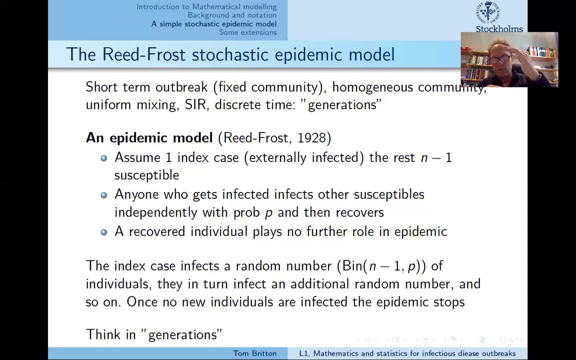 will not increase. It starts increasing in the beginning, but after a while, since there are fewer and fewer remaining susceptibles, it will start decreasing And at the end it will stop. since we have only 1000 individuals, It has to stop at least before generation 1000. 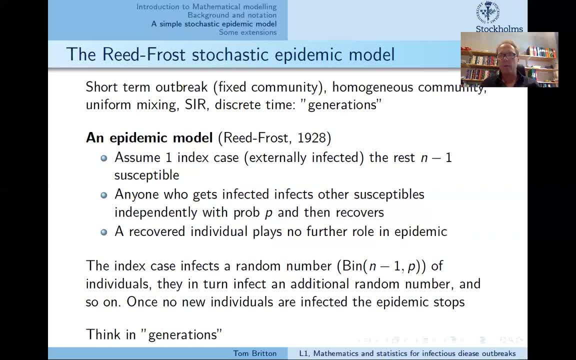 And typically it will happen much earlier than after 1000 generations. So this is the model. It's a random model. It has one single parameter, and that is p, which is the probability to infect a given other individual, And then it has a population size. 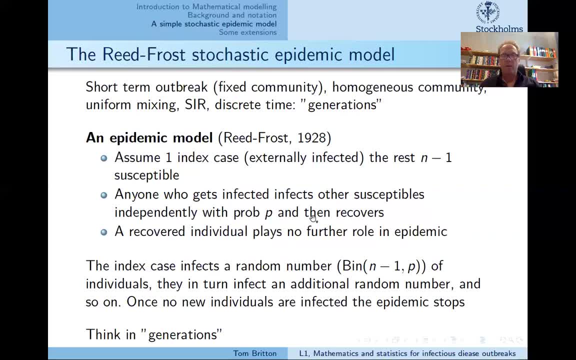 which is called n. Actually, how many you infect in the beginning can be described by a random quantity called the binomial distribution, And the index case infects each with probability p, and there are n minus 1.. So the number of people the index case infects. 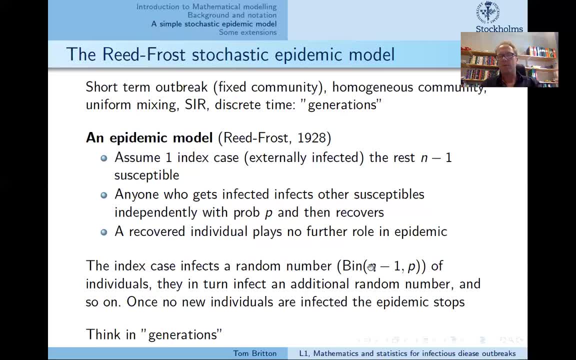 is actually a binomially distributed random variable with parameters n minus 1 and p. But if you don't know probability, that's not very informative, But in case you do, that's some added information. So that is the model. Let's see if we can say anything about this model. 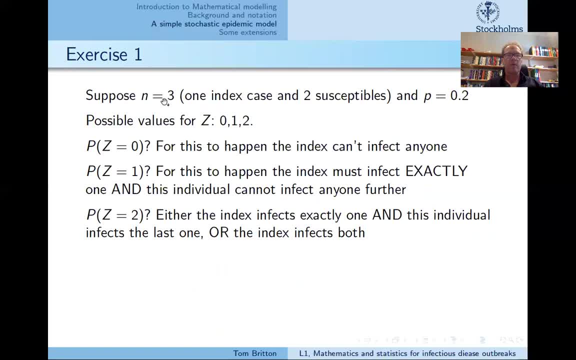 Let's start with a simple case. Suppose we have three individuals only. As I said, we are mainly interested in a large community, but let's start with a small community: Three individuals, One index case and two susceptibles, and let's assume that p is 0.2.. 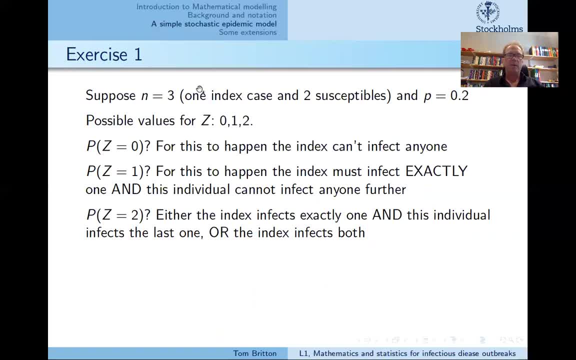 Then how many can get infected? Well, the index case is excluded, so it is these two susceptibles that could either get infected or not. So z can be 0,, 1, or 2.. So what is the probability that z is equal to 0?? 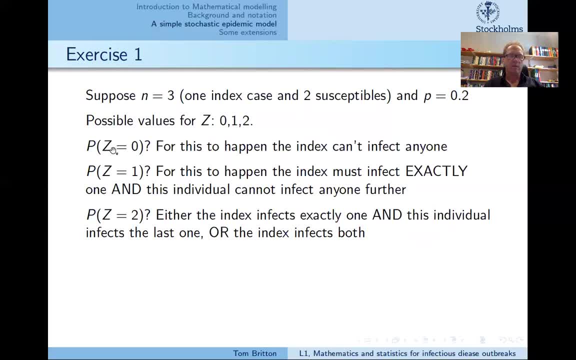 That means: what's the probability that no one gets infected? Well, that happens if the index case does not infect anyone. That's the only way this can happen. What's the probability that one person gets infected? Well, for this to happen, 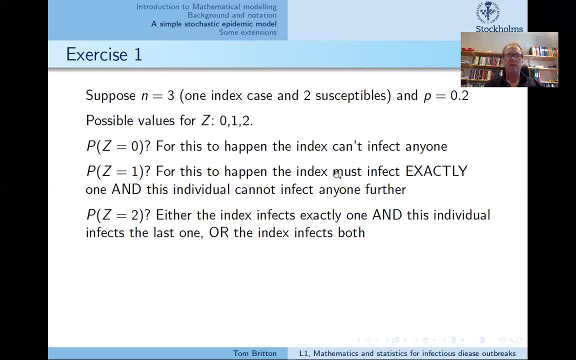 two things must happen. First of all, the index case must infect exactly one person, but also this newly infected is not allowed to infect another one. And finally, what's the probability that both people get infected? Well, that can happen in two different ways. 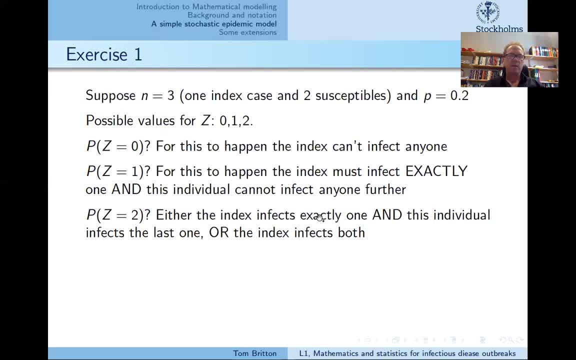 Either the index case infects both, or else the index case infects one and that newly infected infects the other one. So this reasoning gives us actually the following expressions: So the probability that no one gets infected is the probability that the index case 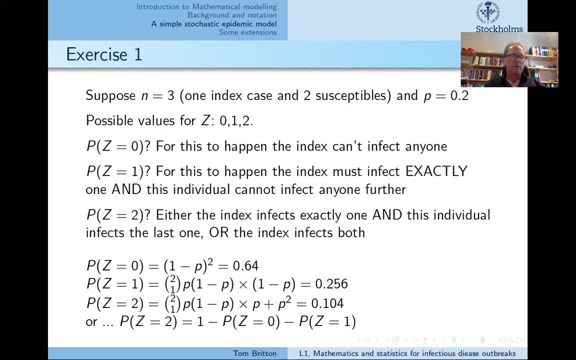 the two coin tosses the index case does both result in non-infection And the probability of non-infection is 1 minus p and since it's two coins, the probability is 1 minus p squared and 1 minus p is 0.8,. 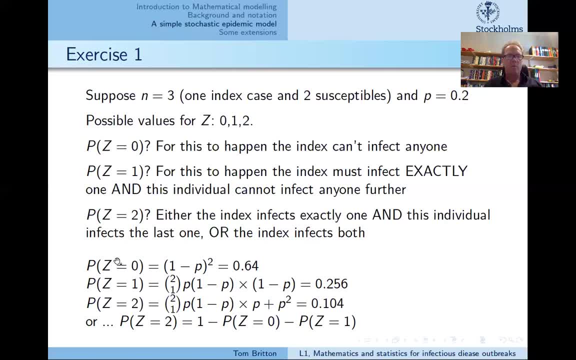 since p is 0.2, so the probability of no one getting infected is 0.64.. The probability that one individual gets infected happens if the index case infects one person and there are two to choose from. so the number of possibilities to select one out of these two. 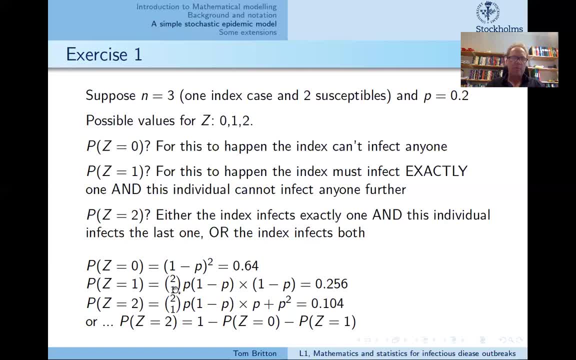 is two. choose one, which is equal to two, of course, and you should infect one of them and not infect the other, but then, as it was said here also, this newly infected person should not infect the final person, and the probability for this is 0.256.. 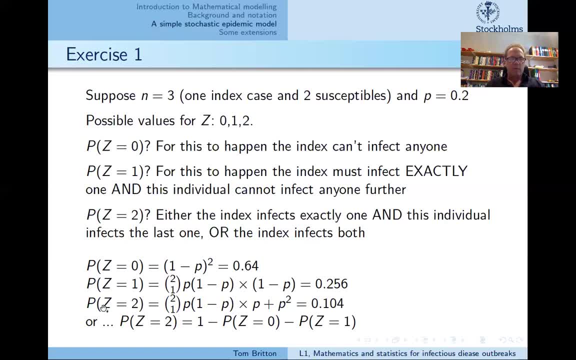 And finally, the probability to infect. that two people get infected happens either if the index case infects one, but then, instead of not infecting the other, he or she must infect the other one, or else the index case directly infects two people. 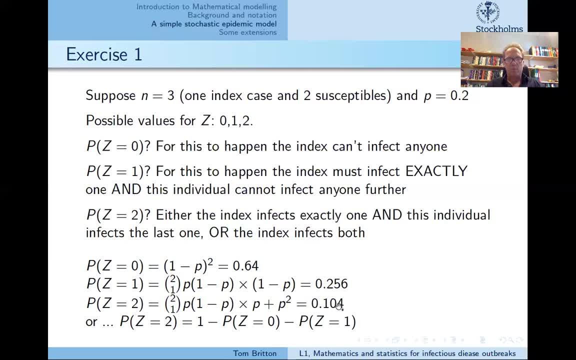 so it's a sum of these two terms, and that is probability. The lazy way would, of course, be to compute the probability that two get infected as 1, minus the probability that zero get infected, minus the probability that one get infected. 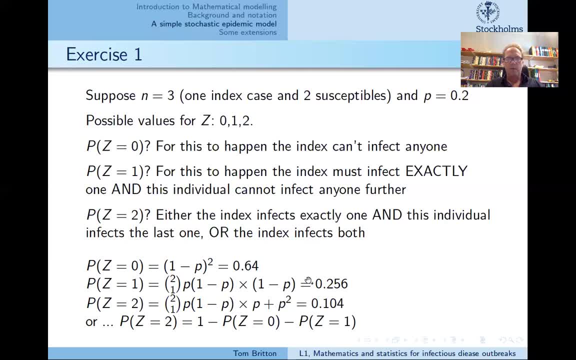 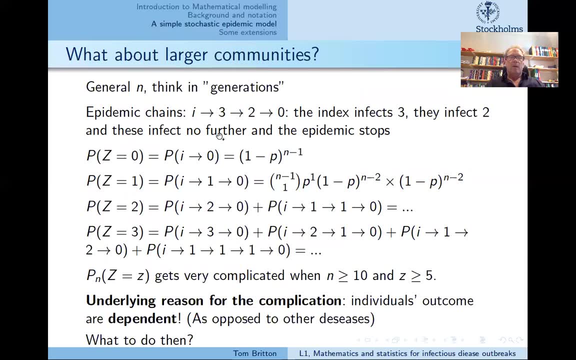 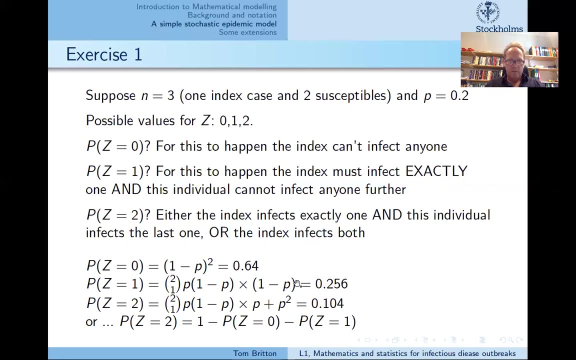 But it's good to do this, and then you can add these to confirm that you get one, and here you actually do Okay, As was sort of described here, in particular here and here, the way to think is in terms of generation. 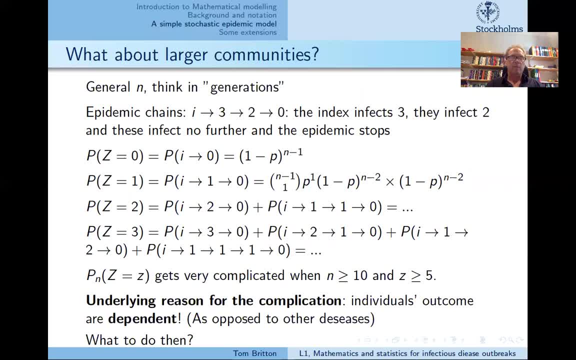 It's quite hard. for a large community, it's very hard to say what's the probability that seven out of 14 get infected. What you should then do is you have to split up the possibilities of seven people getting infected into the different ways at which this can happen. 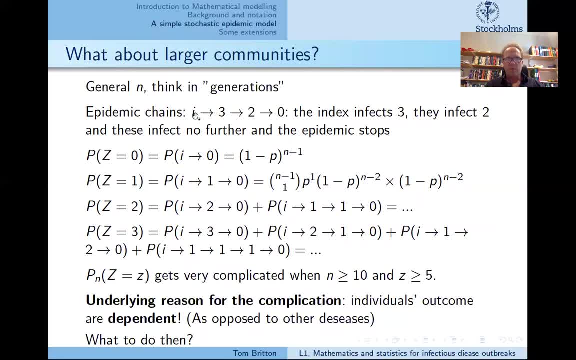 So here is a particular chain of infection. So this chain here means that the index case infects three people. these three people infect an additional two people in the next generation and these two infect no one in the next generation. If you do that, 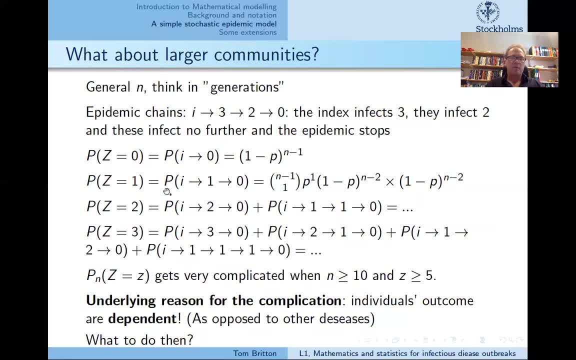 you can write the final outcomes as the sum of the different chains. So the probability that no one gets infected is. the only possibility for that is that the index case infects no one. So that has this probability: The probability that one person gets infected. 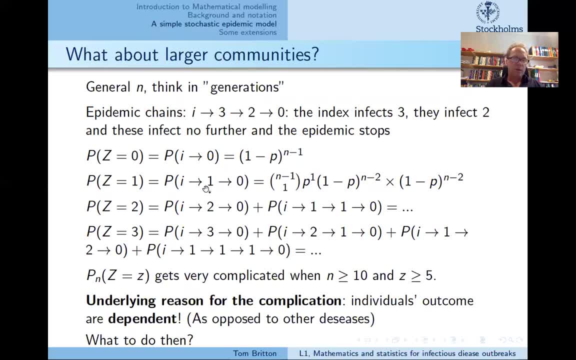 is the probability that the index case infects one and then that this individual infects no one later on. which has this probability in general? How about the two people get infected? Well, that can happen in two ways. Either that the index case infects two. 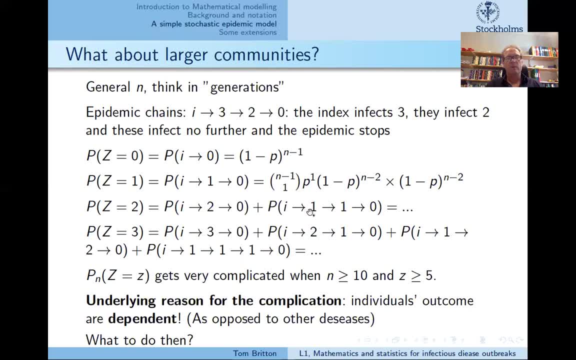 and these two infects no one, or the index case infects one, that person infects another one and that person infects no one. Three: the index case can infect three, then followed by no one. index case infects two. 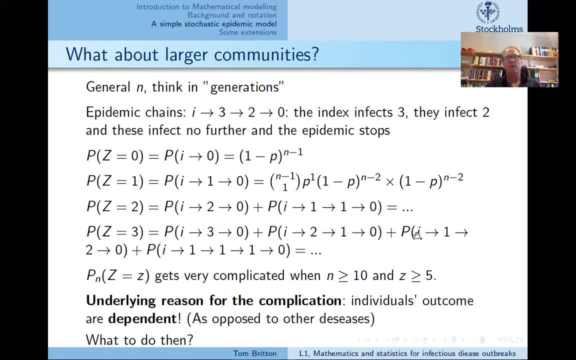 followed by one more, followed by no one, or index case infects one, and then that one individual infects both, and then- sorry- two, and then that one infects no one, Or one, followed by one, followed by one, 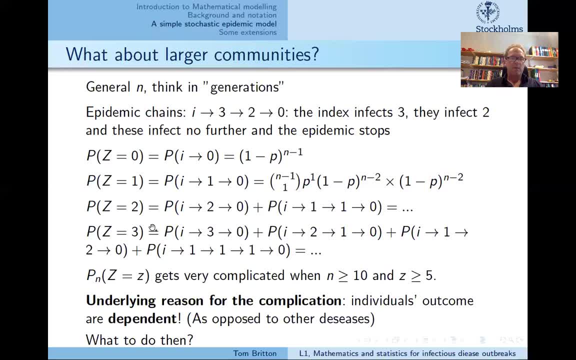 followed by no one. So you can imagine that if you choose a larger number here, the number of possible chains are quite complicated, and actually so are these expressions also. So the probability to compute- this is sorry the way to write this probability- 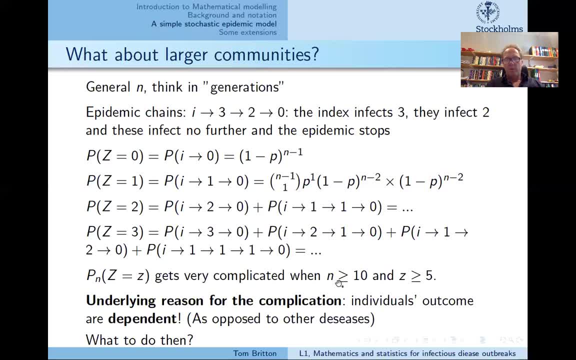 becomes very complicated. if you, let's say, you have a population that's larger than 10, and you want to compute the probability of, let's say, having at least five people getting infected, It would take the probability to have exactly five out of 10,. 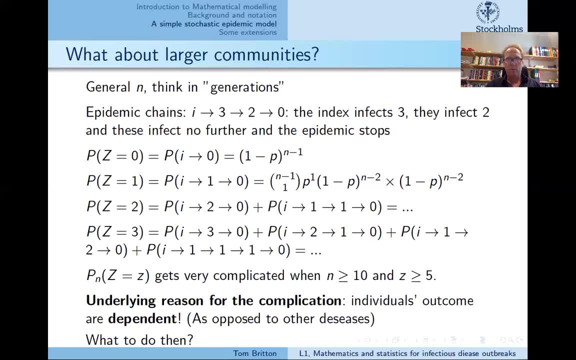 that would take probably about one day to compute- Maybe not one day, but at least several hours. And the underlying sort of why is this the case? It is because who gets infected in the next chain depends on who was infected in the previous chain. 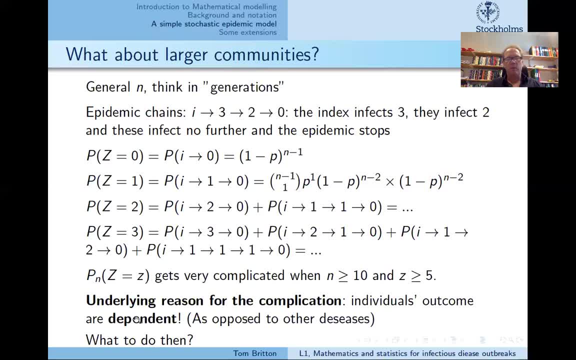 So there are some dependencies, which is not typically the case in most probabilistic situations. Okay, So I defined the model, which was simple and still, the conclusion was that it was very hard to analyze. What's good with that? Well, hopefully there are other ways around this. 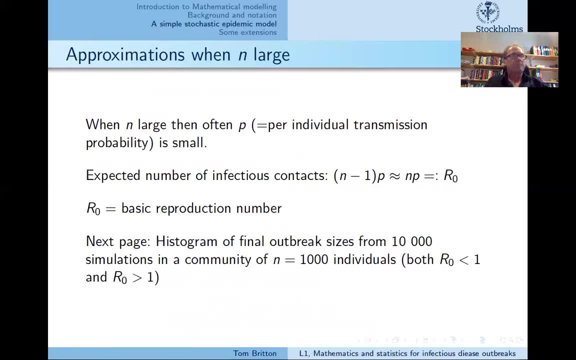 which I will now try to explain. So when N is large, as I will assume, you typically assume that P is small, Because, let's say, if you consider the spreading of a disease in Stockholm, you have maybe 1.5 million people. 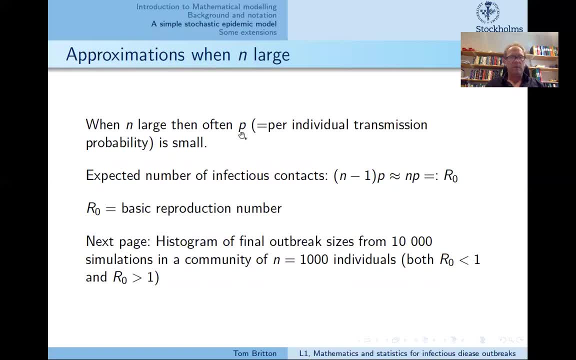 What's the probability to infect a random guy in Stockholm? That's a very small probability. So the average or the expected number of people that you infect is N times P Or, if you want to be really rigorous, the expected number that the index case infects. 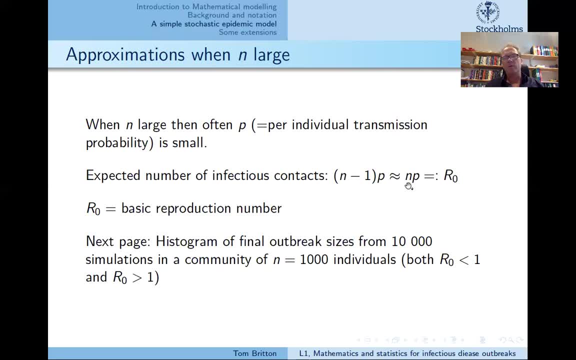 is N minus 1 times P, But in a large community that's more or less N times P. This quantity is called the basic reproduction number, denoted R0.. That's something that no one knew about half a year ago, but now. 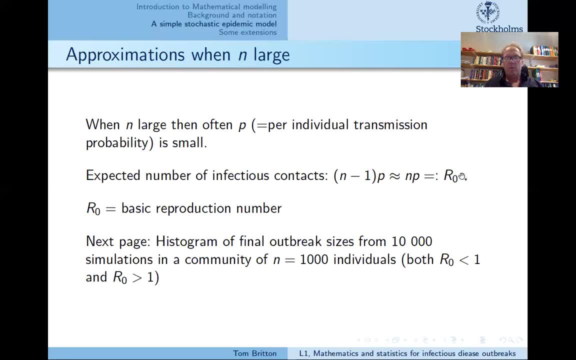 many people in Sweden or in the world have heard about the basic reproduction number due to the COVID-19 pandemic. So what I've done on the next slide is that I have simulated an epidemic in a community of 1,000 individuals. 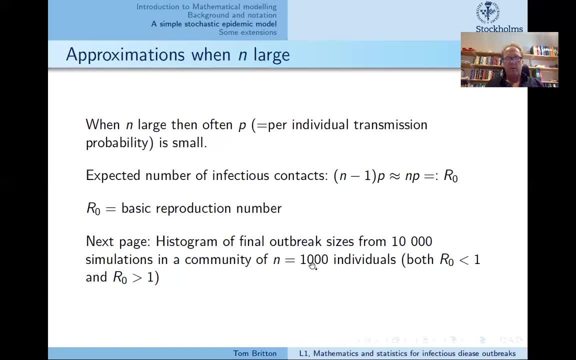 So I started with one person being infected and 909 people, 999 people being susceptible. I simulated, so maybe three got infected, next generation, maybe seven, maybe 15,, maybe 29, and so on until it stopped And the only thing I kept 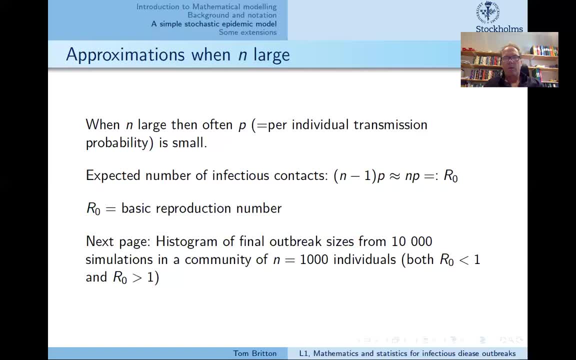 was how many that got infected. So maybe the result was that in the first simulation maybe 577 people got infected, so I keep that 577.. And then I repeated this 10,000 times and I stored how many got infected. 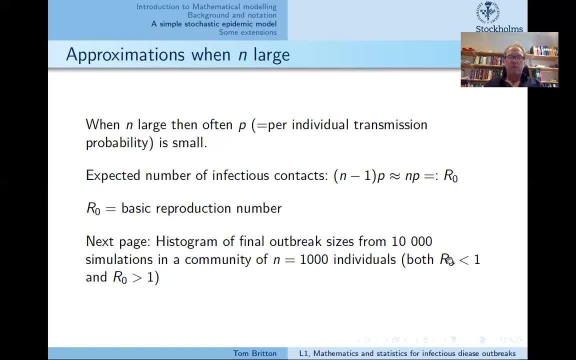 And I did it for two possible two values of R0. The first one was smaller than one and the second one was larger than one. And now on the next slide comes a histogram showing how many people got infected. and the first histogram is for: 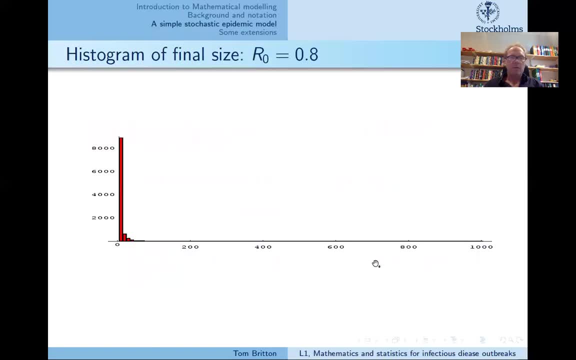 when R0 is 0.8.. So when R0 is 0.8, we see that of the 10,000 simulations, all result in very small outbreaks. We see that nearly all are between 0 and 10 people get infected. 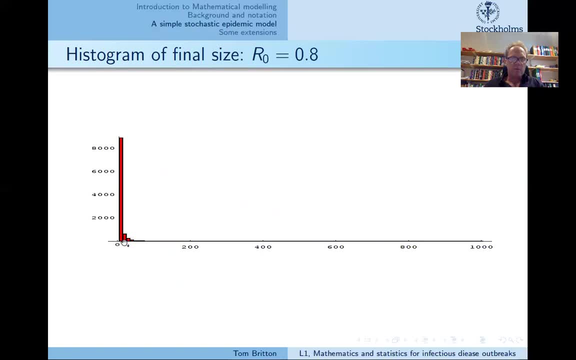 a few are between 10 and 19 infected, and I think the largest one had 57 infected or something like that. So all are very small outbreaks when R0 is 0.8.. And then I did the same thing when R0 is 1.5.. 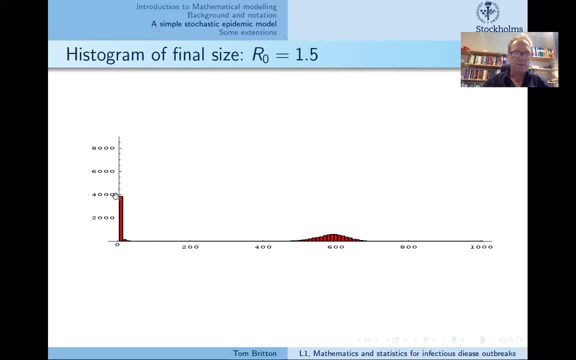 And then we see that there are still some small outbreaks, actually close to four, or actually, if you would add this, it would be slightly more than 40% of the outbreaks that are small, and then the rest, which should be slightly less than 60%. 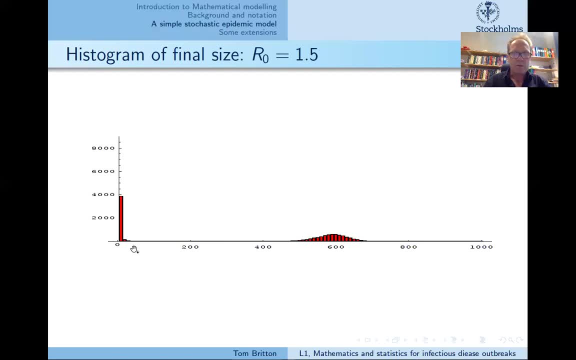 are large, But the large ones, they are not distributed anywhere between 0 and 1,000, which is the largest possible value that can get infected. They seem all to be concentrated around 600. And it looks like the peak of this mountain. 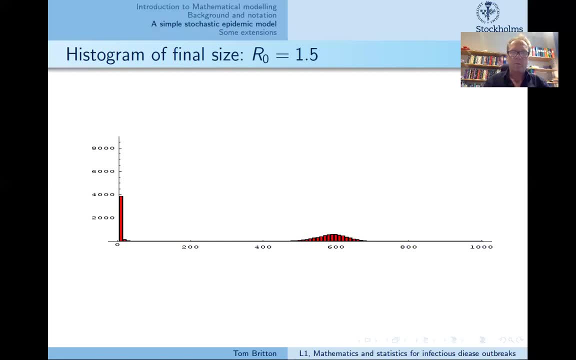 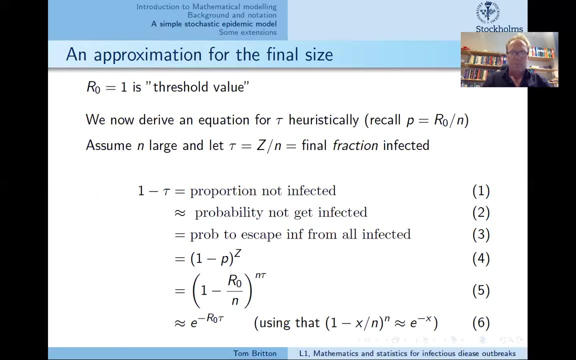 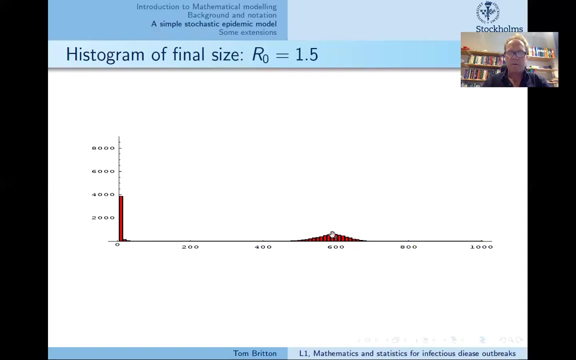 is slightly below 600.. So that is perhaps surprising, And now I will try to explain using heuristics. using heuristics, we can actually explain why the fraction getting infected- in case you do not have a small outbreak- why they are concentrated around 60%. 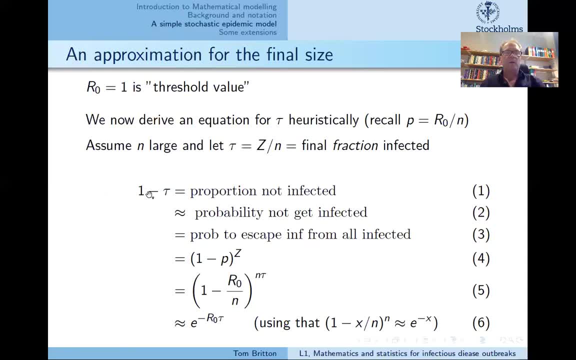 And here comes the explanation. So we fix R0.. And we let tau be the final fraction getting infected. So tau is the final fraction getting infected. Recall that p times n was R0.. So p is equal to R0 divided by n. 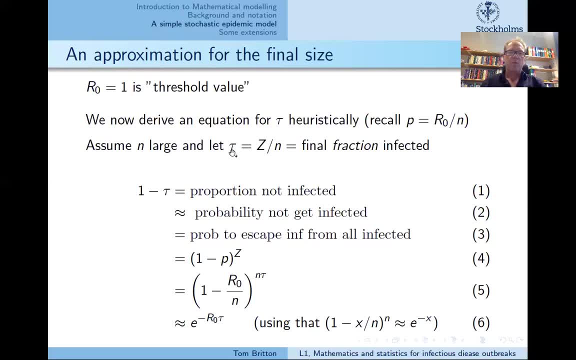 And we assume that n is large And tau is the final fraction getting infected, So it is the final number divided by n. So if tau is the fraction getting infected, then 1 minus tau is the fraction not getting infected And the fraction or the proportion. 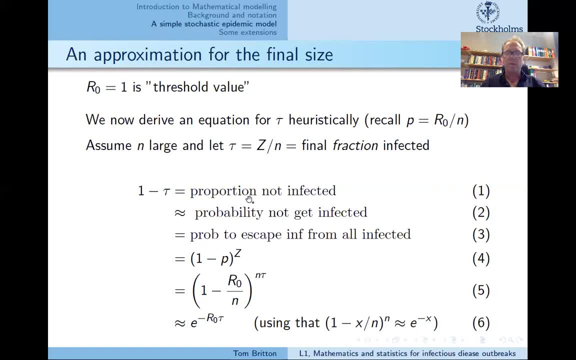 not getting infected. that is more or less the same thing as the probability not to get infected And the probability not to get infected, if you think about how I described the model, that is the probability that you escape infection from all infected people. 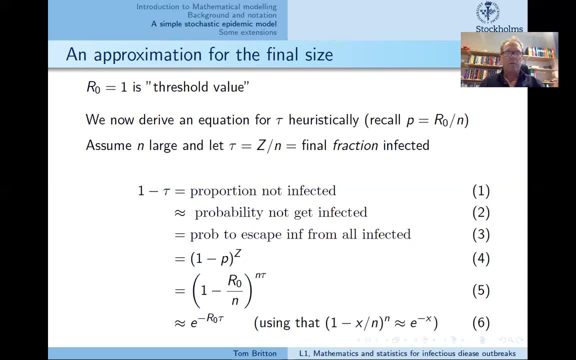 meaning that you avoid getting. you avoid when the infected people toss their coins to you. you avoid infection from all of them. So you avoid infection from all the z people getting infected. That is the probability to escape from infection. Now I just replace p. 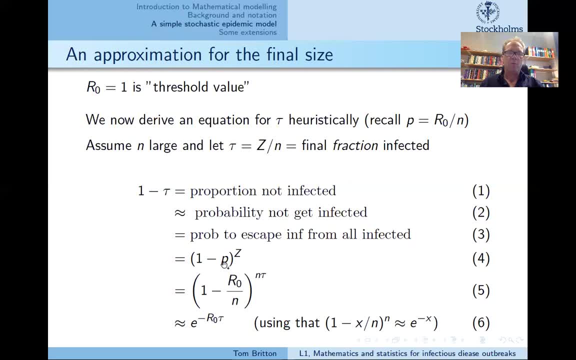 by R0 divided by n, because p was small And R0 was, let's say, 1.5.. So R0 divided by n is small, And I also replace z by n times tau. So z is equal to n times tau. 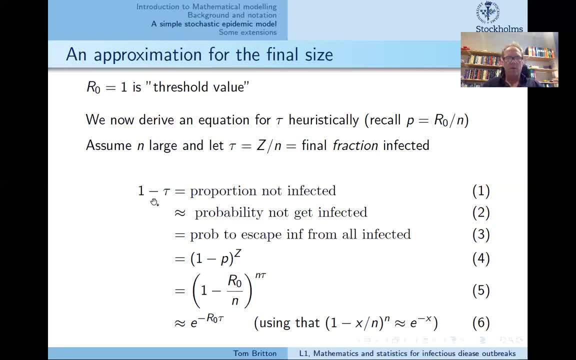 So then we see that we have an equation which says that 1 minus tau is equal to parenthesis, 1 minus R0 upon n end of parenthesis, raised to the power n times tau. And then I think it is shown in the first course and perhaps possibly even in: 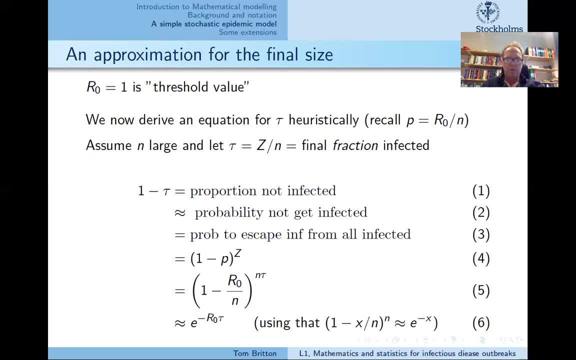 a later course in high school mathematics that if n is large, this expression here is very close to the exponential function evaluated at minus R0 times tau. Using this fact that 1 minus x over n raised to the power n is more or less the same thing. 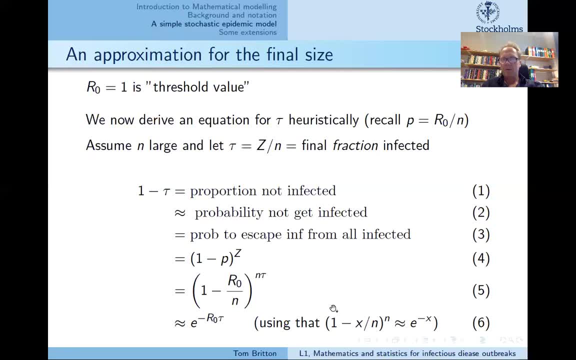 as e to the minus x, in the sense that, as n tends to infinity, this expression converges to that expression. This you have to trust me. If you haven't seen it before, you simply have to trust me that this is the case. So our equation says: 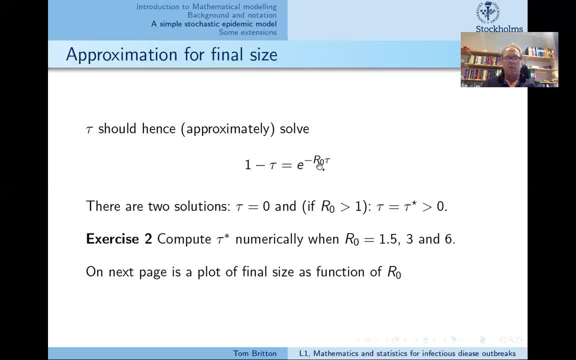 that 1 minus tau is equal to e, to the minus R0 tau. So this is an equation for tau, because R0 was given. So let's say that R0 is 1.5. then you can actually solve this equation numerically. 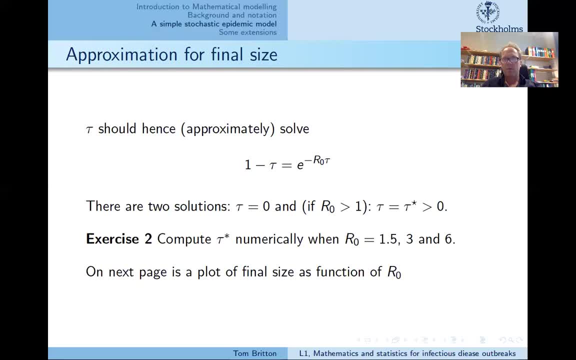 There is no explicit solution, but it has a solution which is easily solved numerically. tau equals 0 is always a solution, agreeing with this that it is possible that hardly anyone gets infected. but then if R0 is larger than 1, there is a second solution. 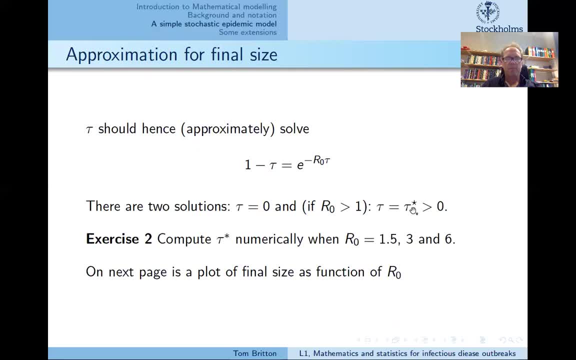 which we call tau star. So one exercise that you should try to do yourself is to solve this equation numerically for a couple of different values of R0. Let's say 1.5,, 3 and 6.. On the next page, 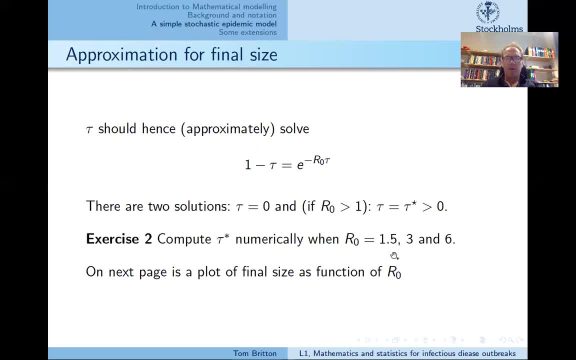 I don't solve it for these three, but I solve it for, let's say, for all values of R0. So it will be a curve on the next slide. it will be the curve how many people that get infected as a function of R0. 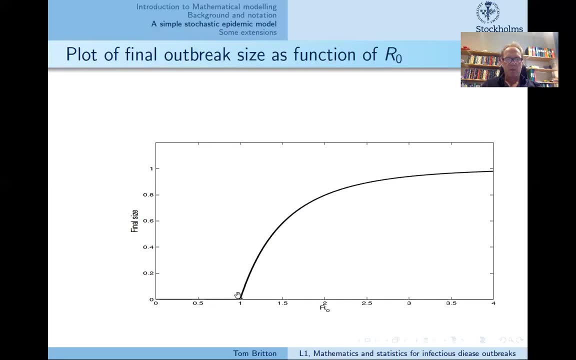 And here is the curve. So we see that if R0 is smaller than 1, no one gets infected, or a negligible fraction gets infected, whereas if R0 is larger than 1, we see that some positive fraction gets infected And if R0 is 1.5. 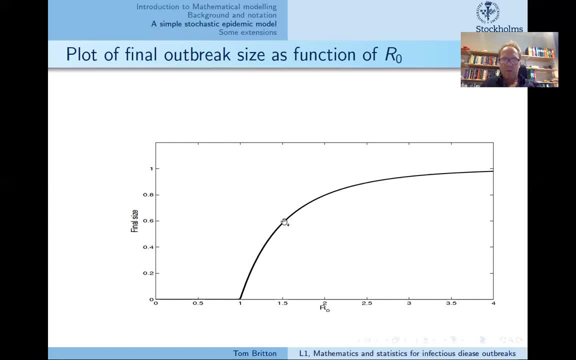 we follow this axis up here and I know it doesn't show exactly, but I know that the numerical solution is 0.583. so this says that if R0 is 1.5, close to 58% will get infected, and this agrees quite well with this. 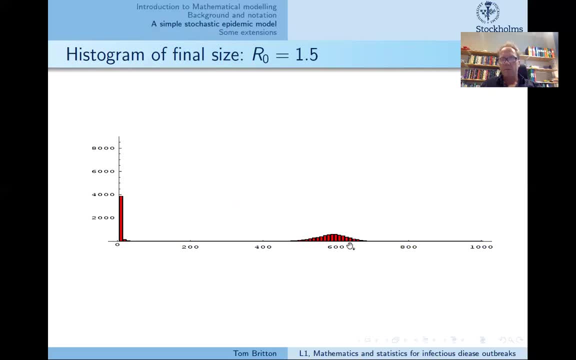 Of course there is some randomness, since it's a stochastic model in a finite population. If I would have done the same thing but would have taken a population size of 10,000, so we would have 10,000 here and here it would say 6,000. 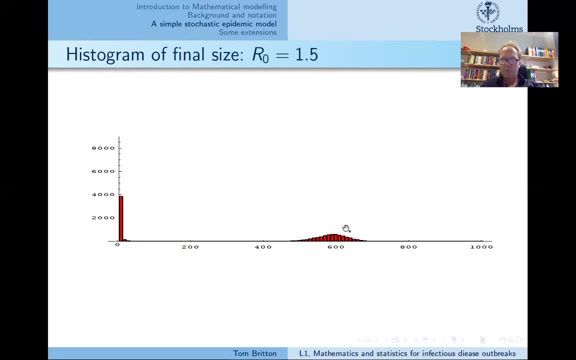 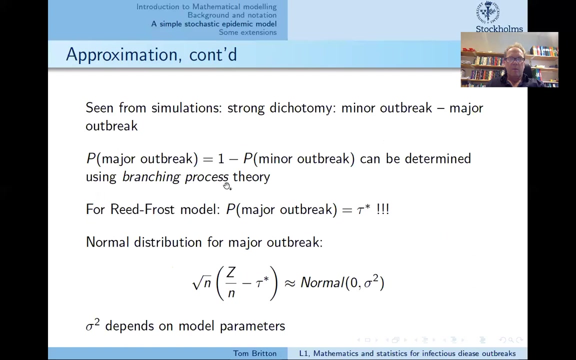 then it would have been a mountain which was much more peaked around 58%, and if we would have taken 100,000, it would have looked like one single bar around 58%. So what are the conclusions? Well, it was clear from the simulations. 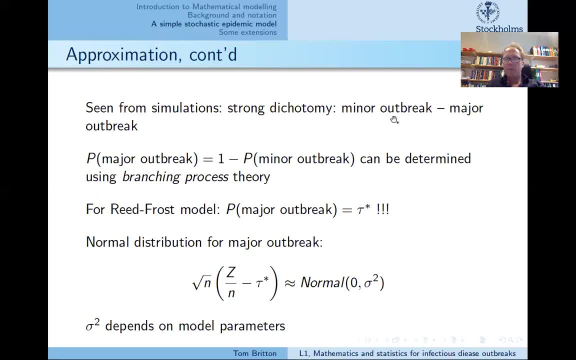 that there is a strong dichotomy: either you have a minor outbreak or, if the basic reproduction number is larger than one, you have a major outbreak. Why does it matter that R0 is bigger than one? Well, probably you can understand that R0 is how many on average? 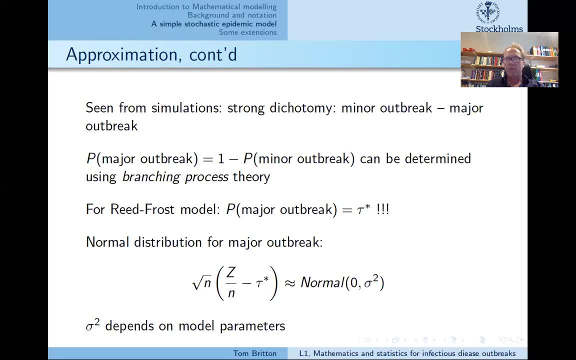 you infect in the beginning, when nearly everyone is susceptible, and if you, on average, infect less than one person, then of course you will not have a big outbreak, whereas if you, on average, infect more than one person, then there is a chance of having a big outbreak. so that is why R0 equal to 1. 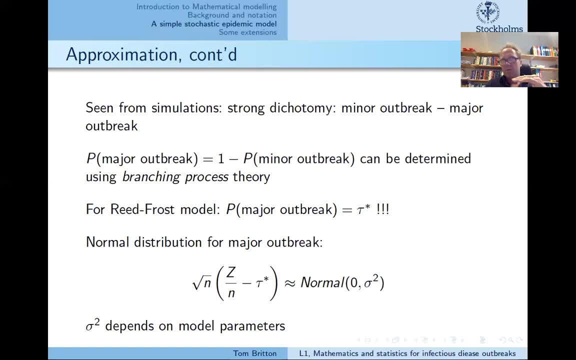 is, let's say, a threshold. if R0 is below 1, there will be no big outbreaks, whereas if R0 is above 1, you can have a big outbreak. I did not talk about what is the probability of an outbreak, although you can, of course, guess this from this simulation. 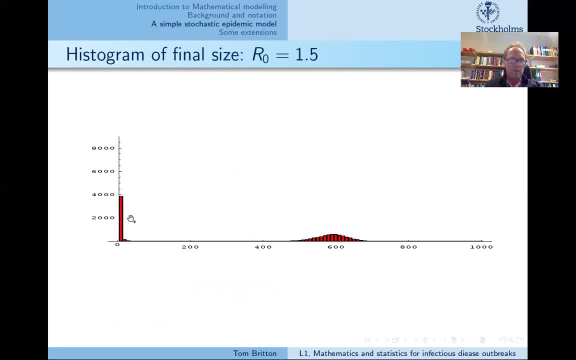 it looks like the probability of an outbreak is slightly above 40%. sorry, the probability of a minor outbreak is slightly above 40%, meaning that the probability of a large outbreak seems to be just below 60% and, in fact, for this model, the probability of an outbreak 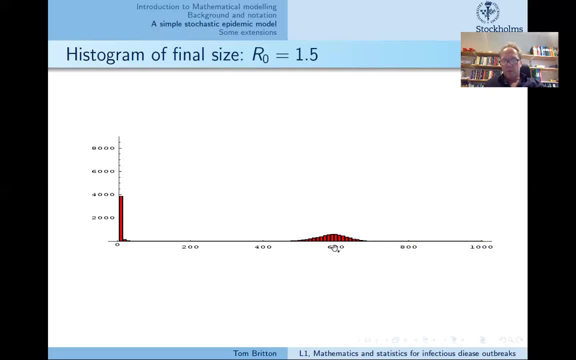 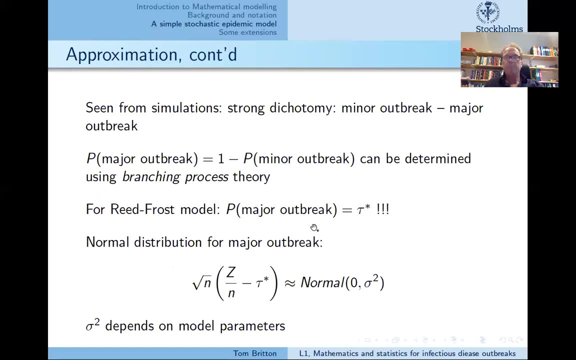 is actually equal to the size of the outbreak, which is something that can be proved mathematically. we are not doing this in this course, of course. You can actually show more well. first of all, the probability of a major outbreak is also the size of the outbreak.